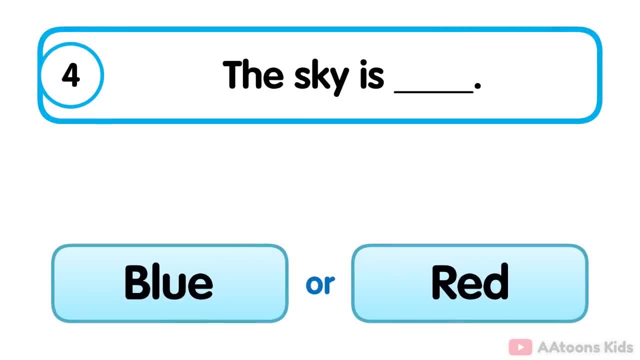 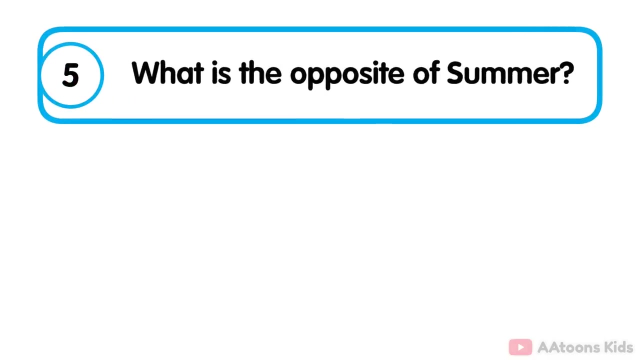 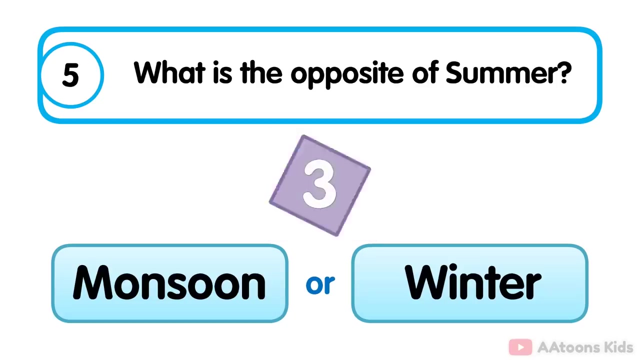 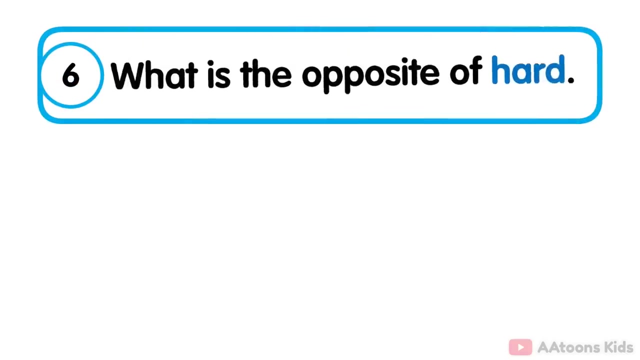 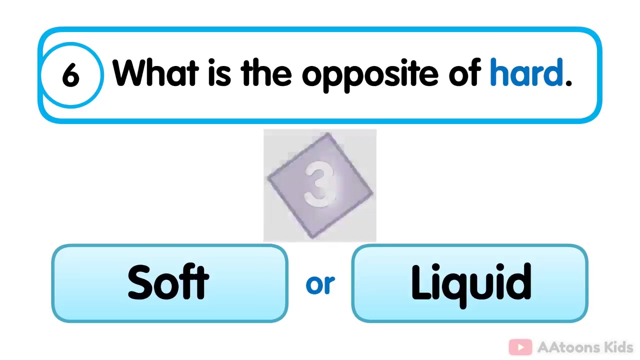 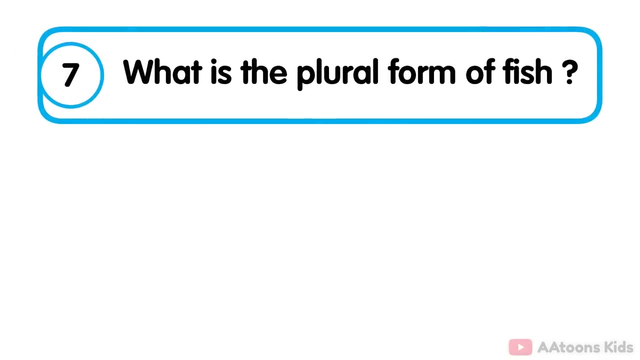 Blue, The sky is blue. What is the opposite of summer: Winter? The opposite of summer is winter. What is the opposite of hard- Soft? The opposite of hard is soft. What is the plural form of fish? Fish, Fish. 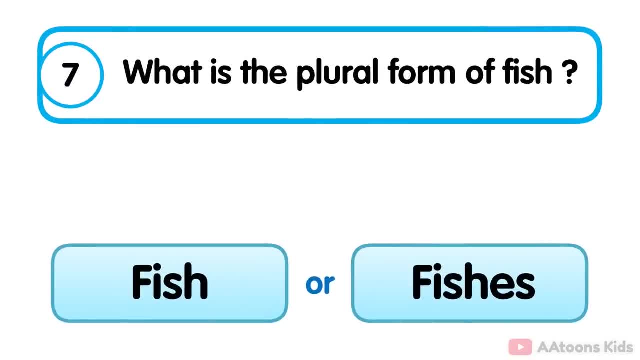 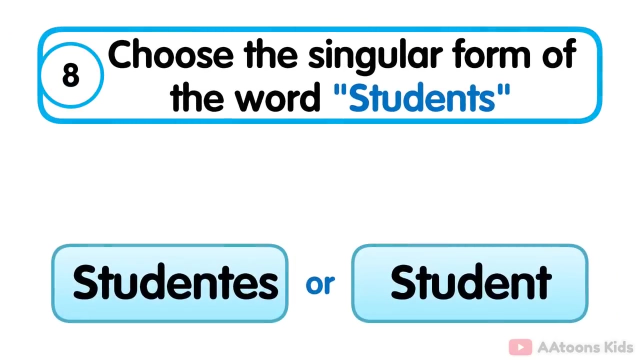 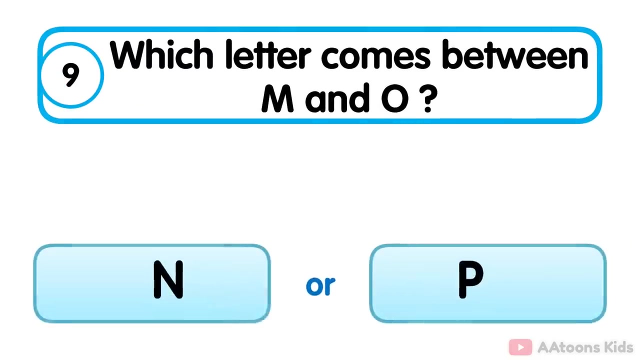 Fishes. Simply add the es in fish, So the plural form of fish is fishes. Choose the singular form of the word a student. simply remove the s from students, so a student is the singular of students. which letter comes between M and O? 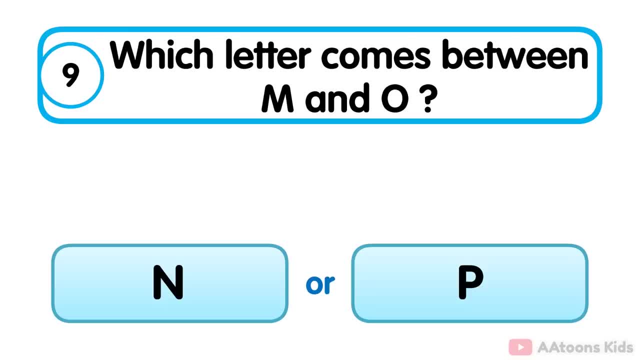 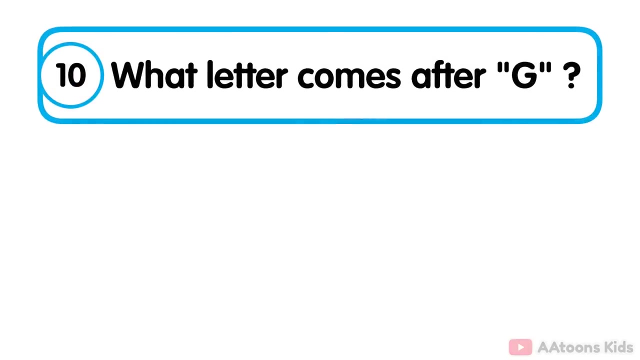 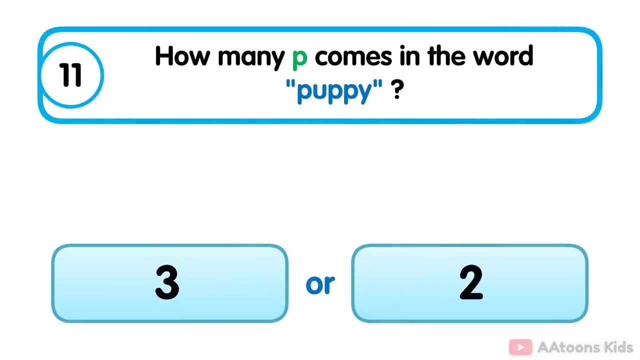 in the letter in comes between M and O. what is the meaning of letter M and O? which letter comes between M and O? which letter comes between M and O? what letter comes after G? letter H comes after letter G. how many P comes in the word puppy? 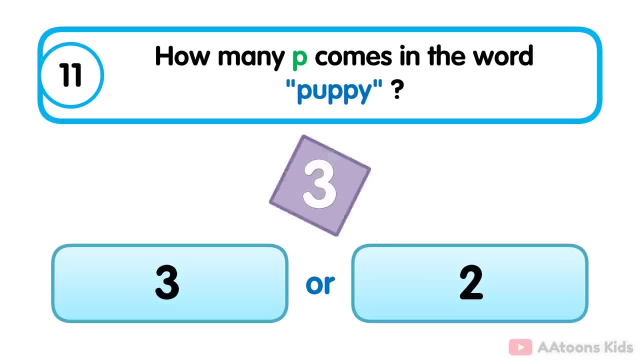 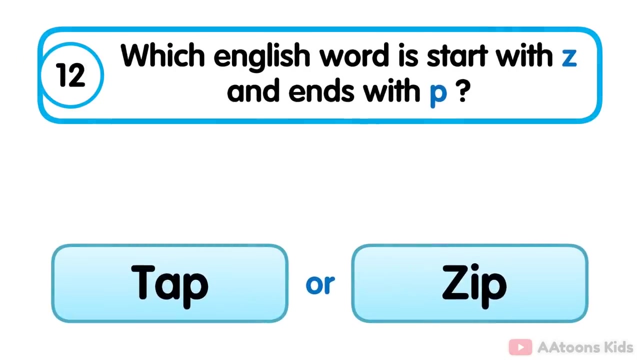 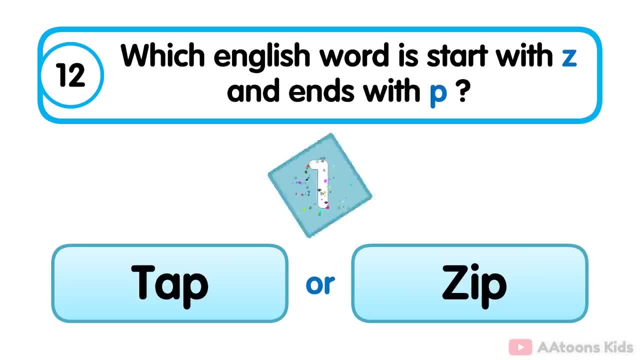 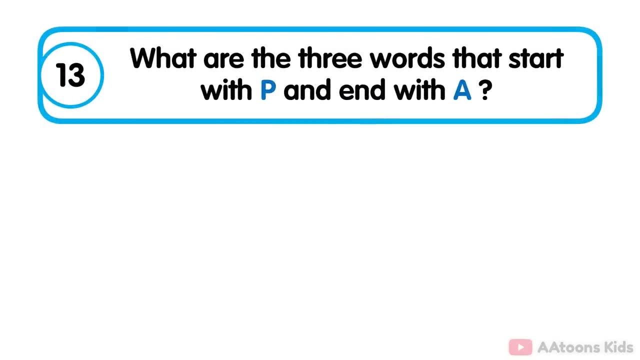 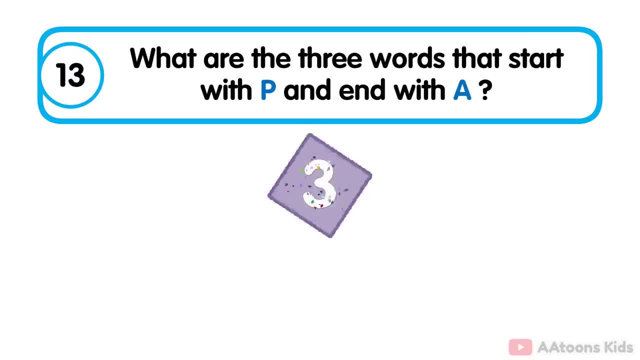 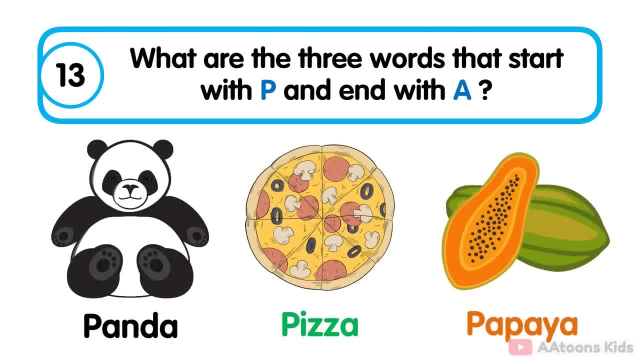 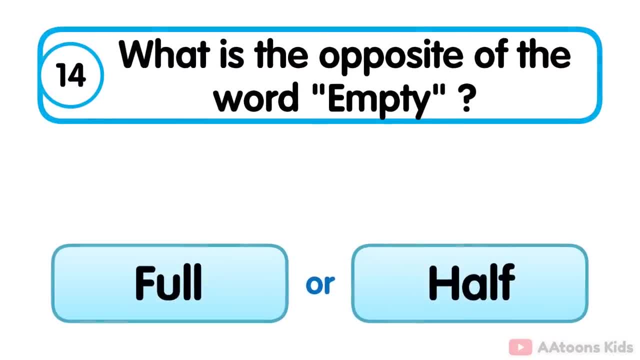 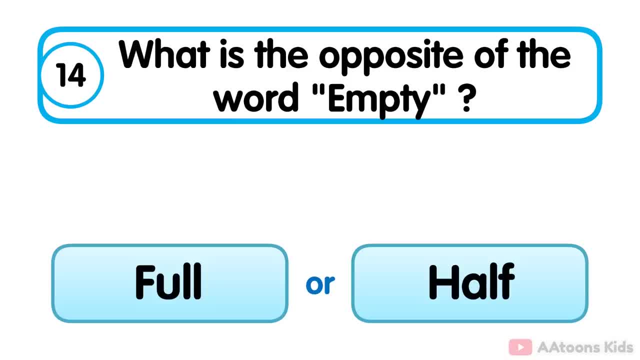 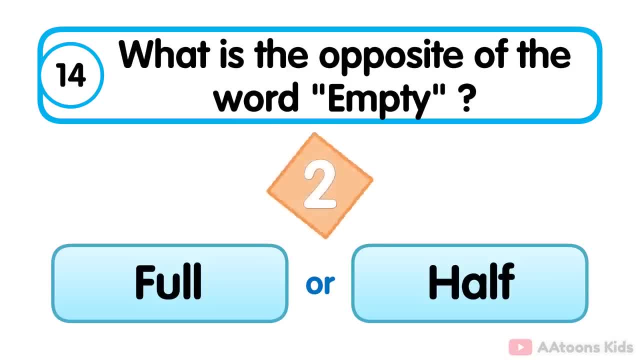 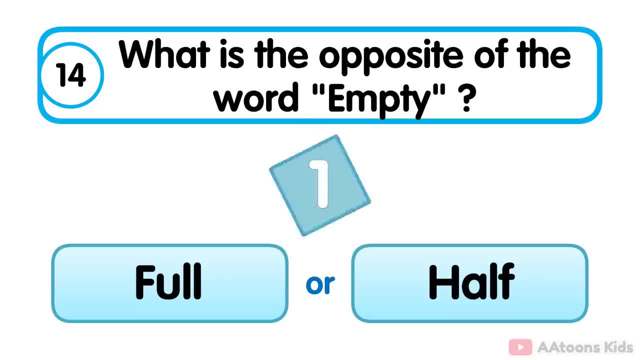 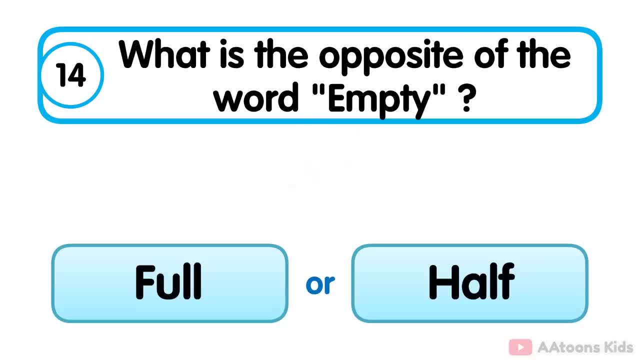 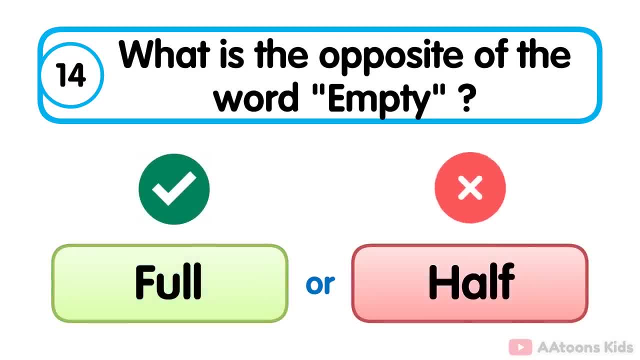 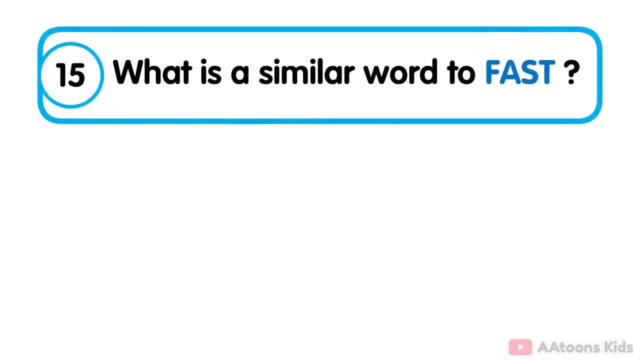 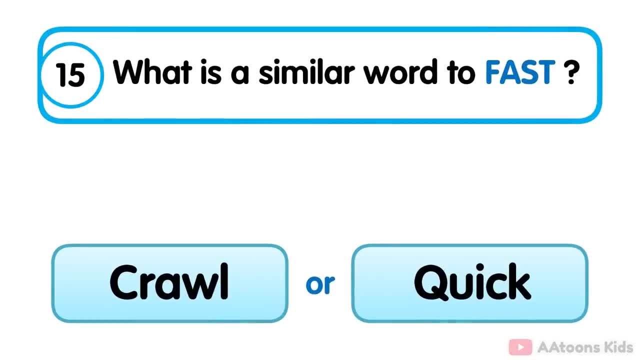 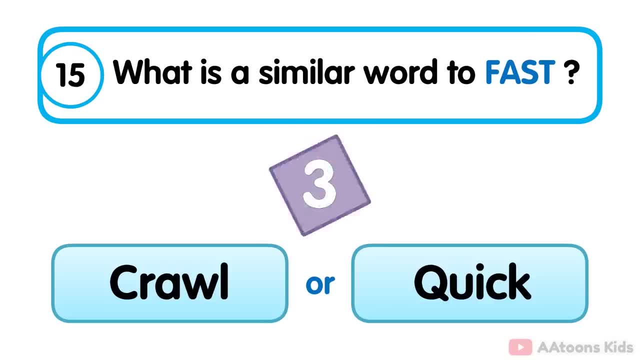 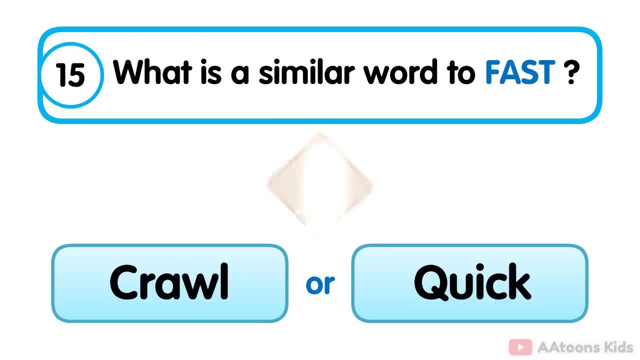 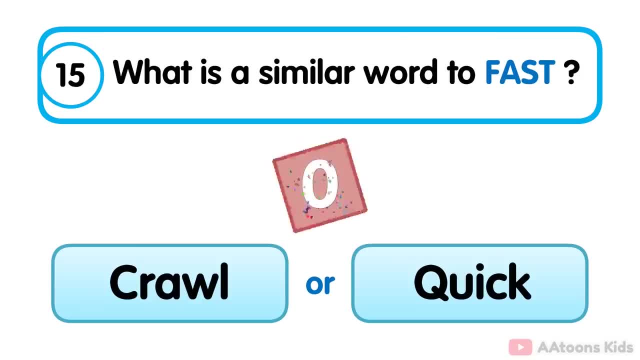 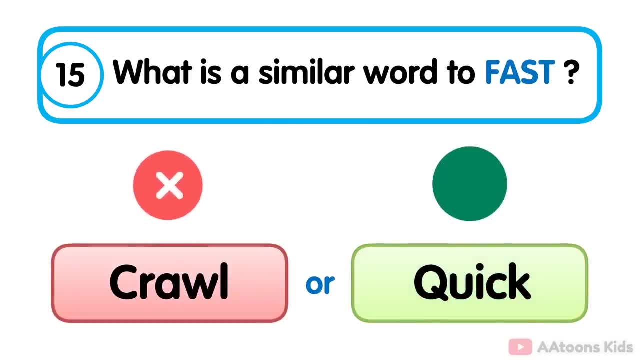 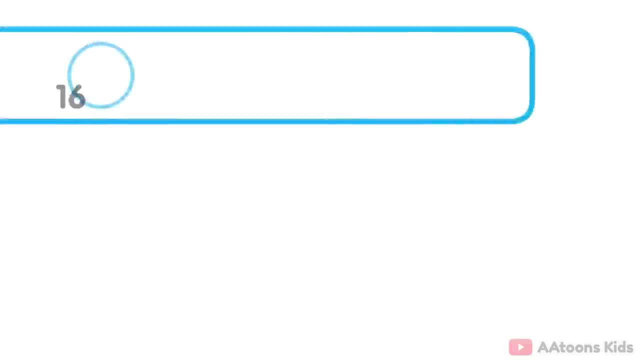 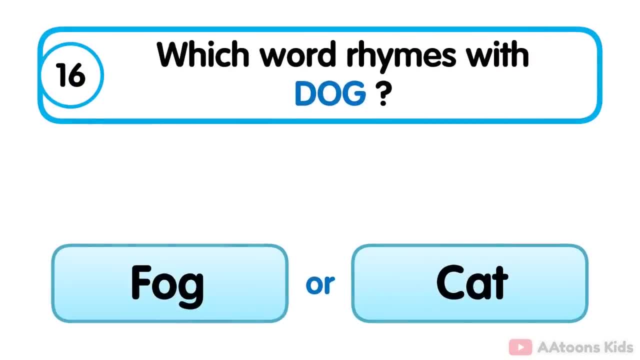 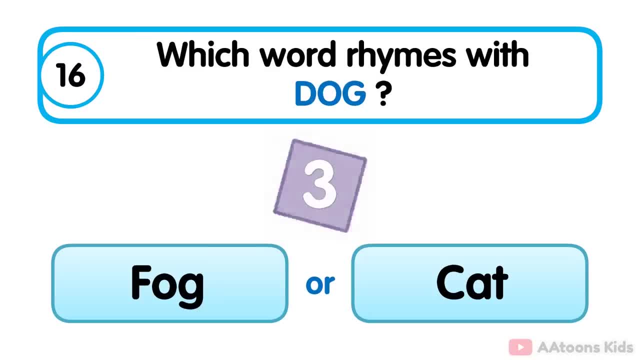 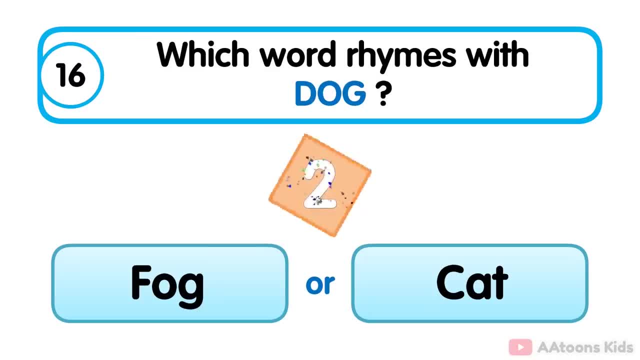 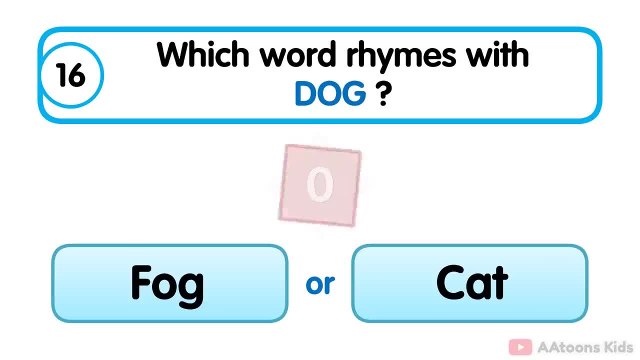 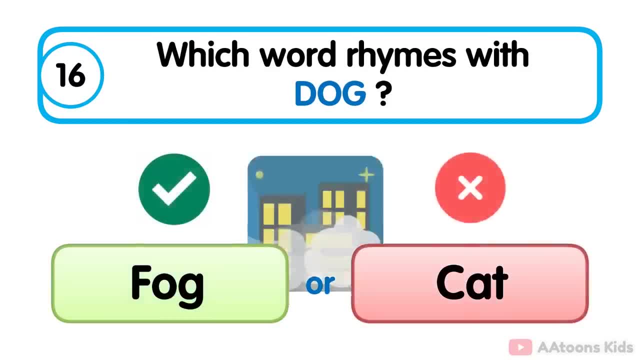 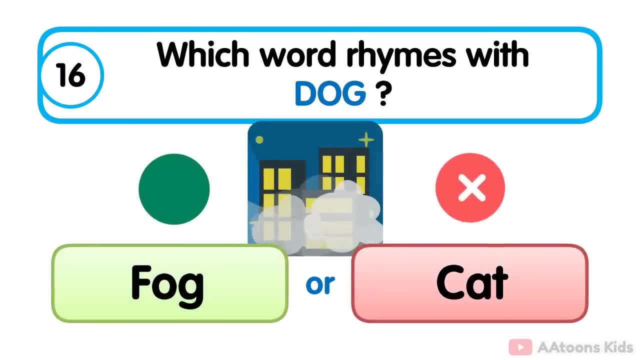 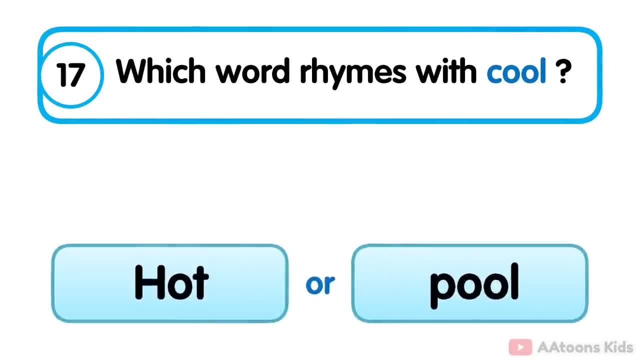 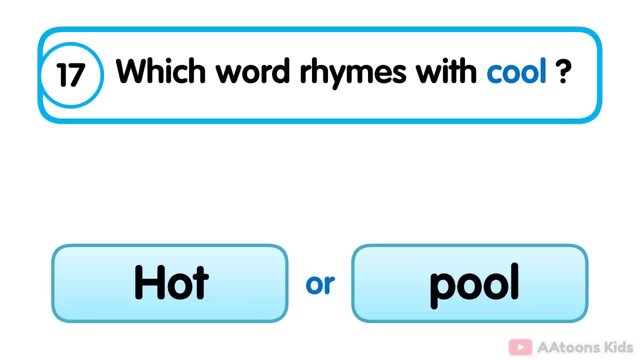 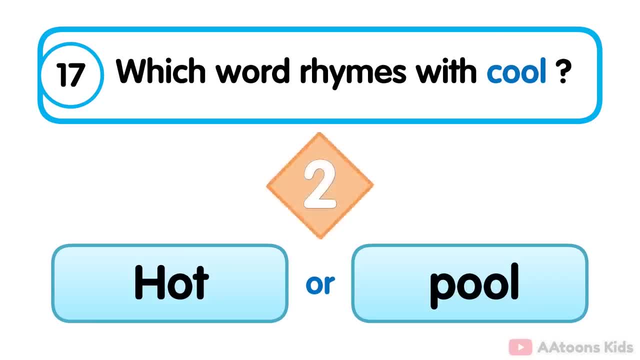 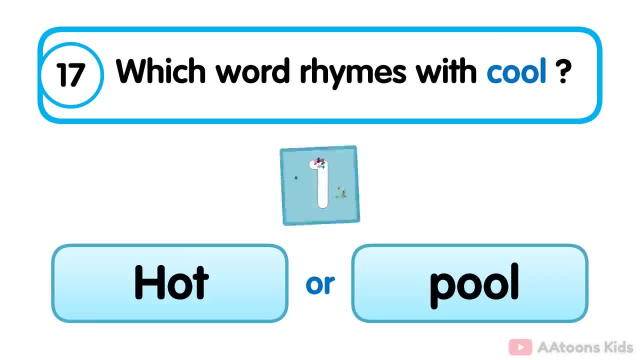 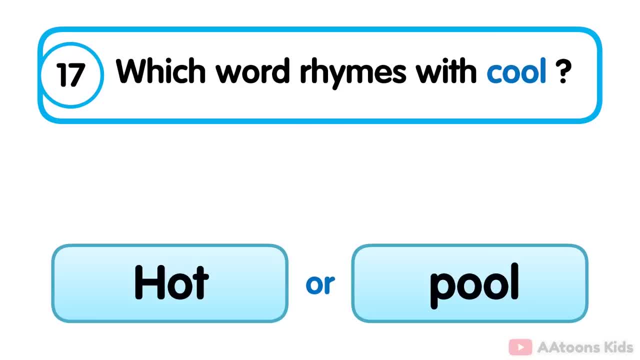 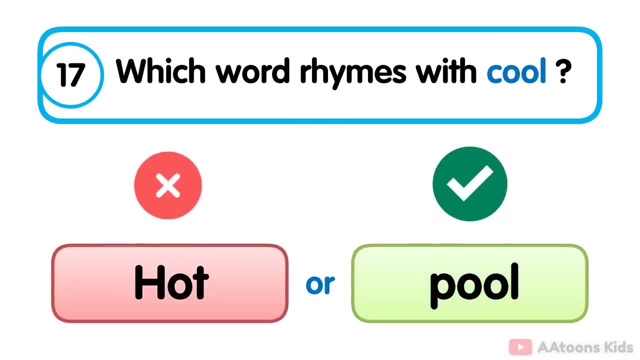 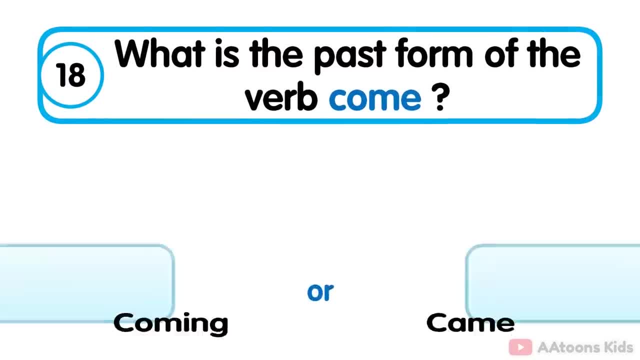 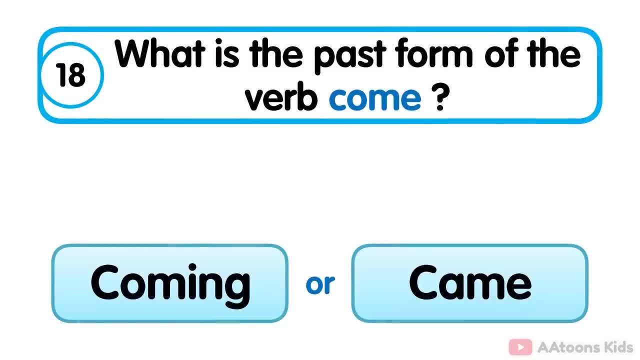 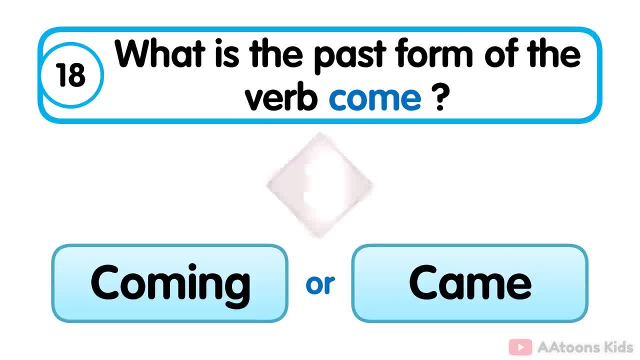 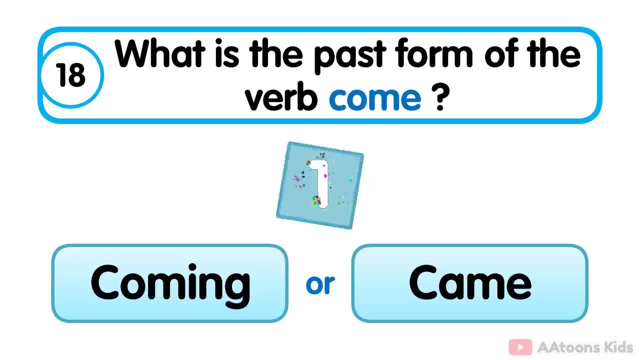 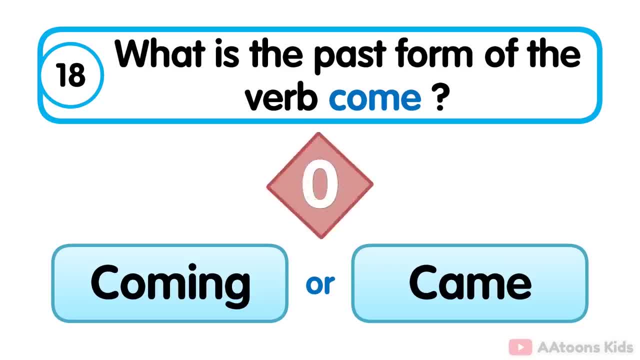 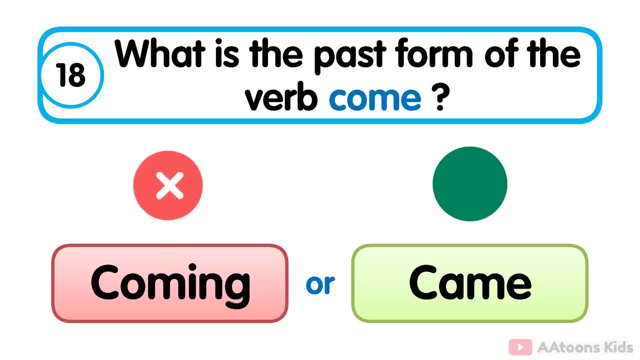 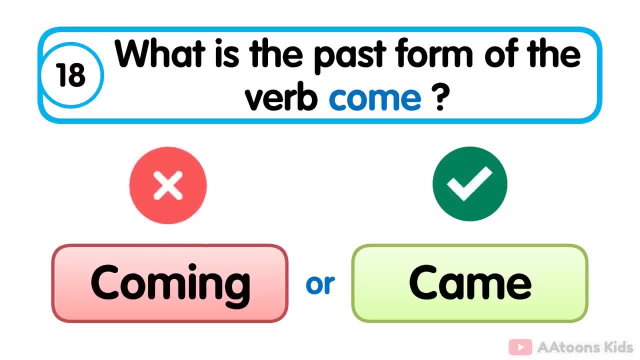 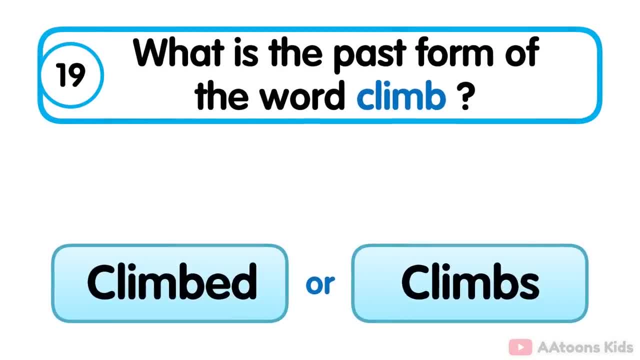 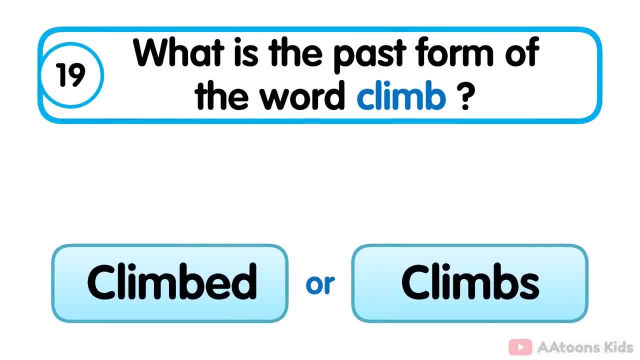 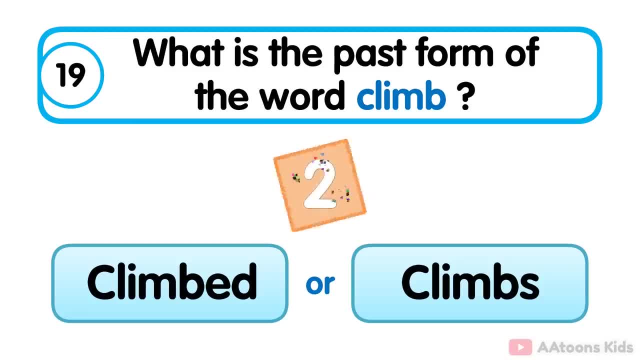 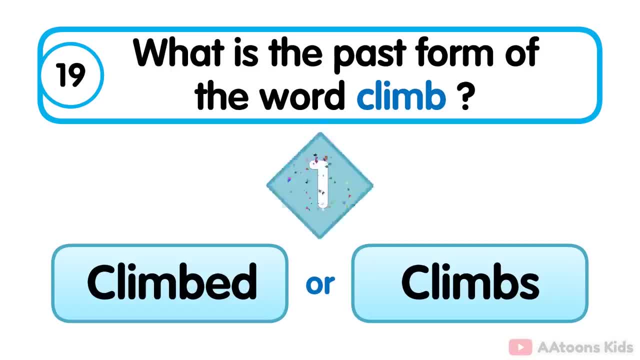 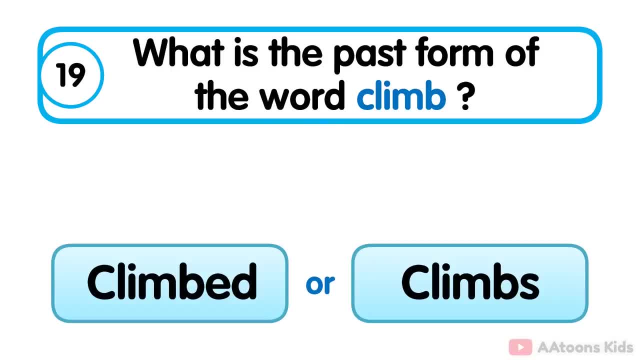 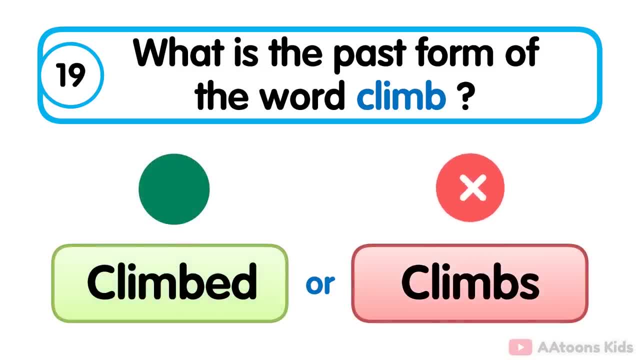 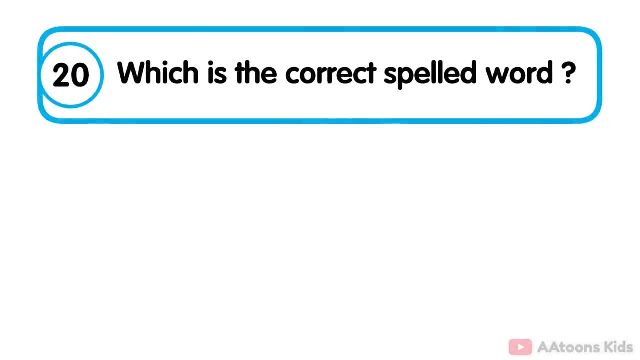 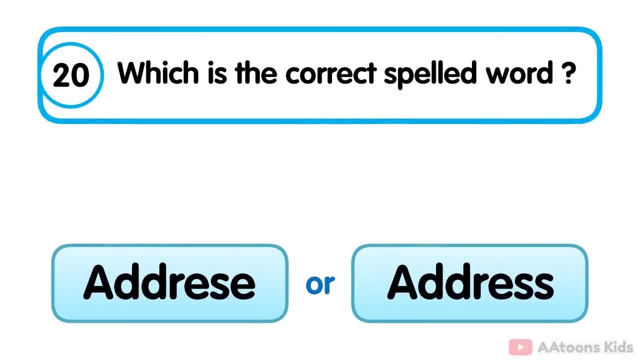 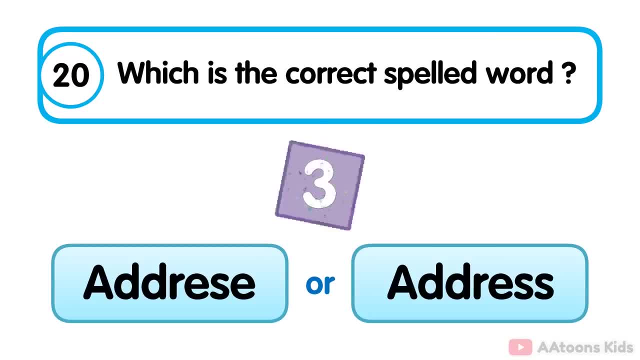 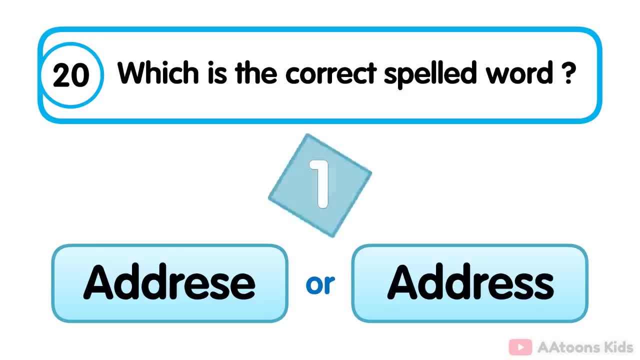 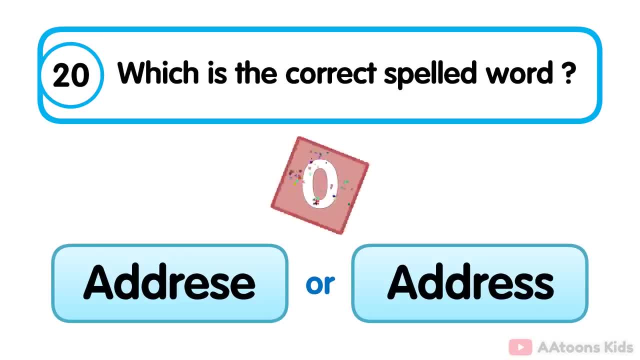 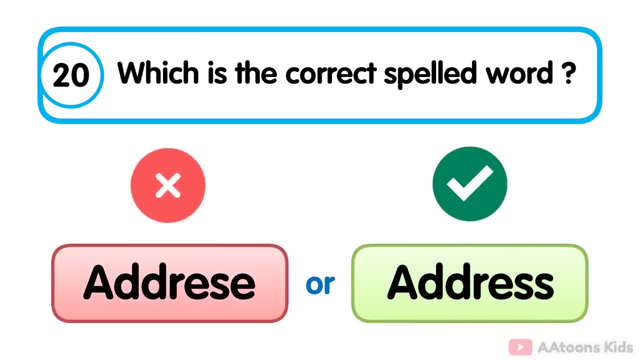 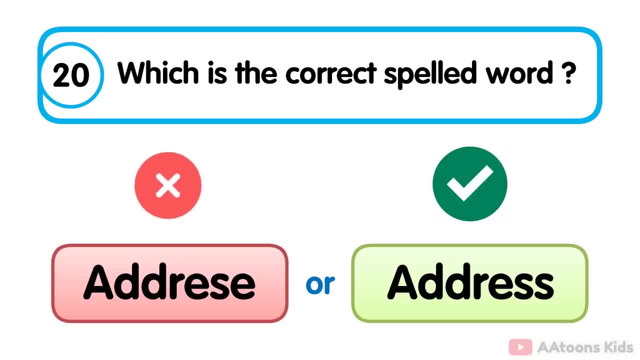 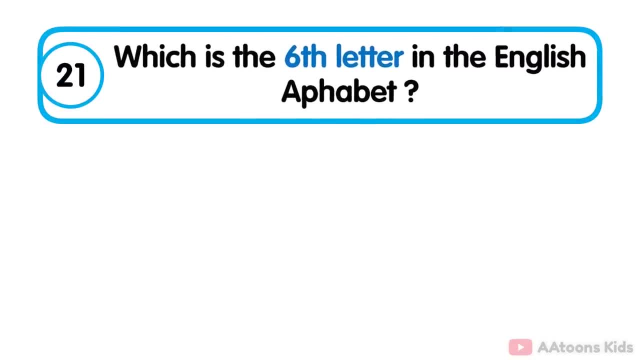 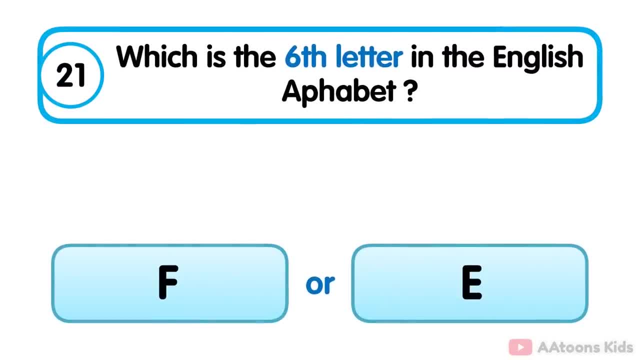 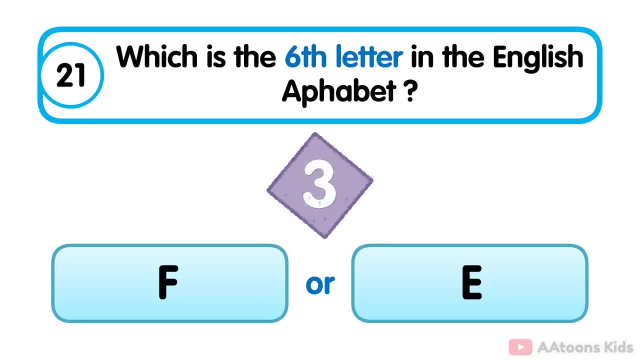 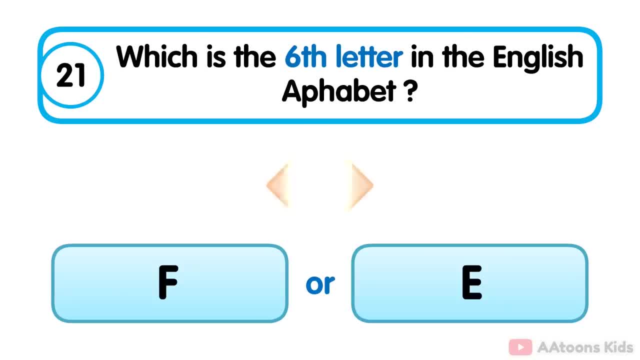 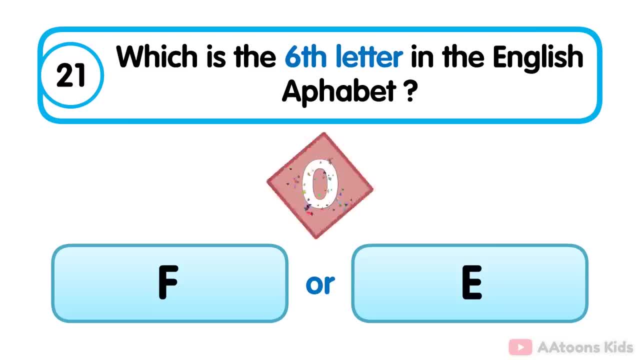 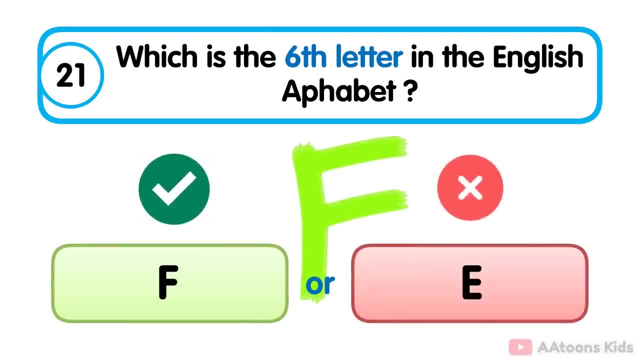 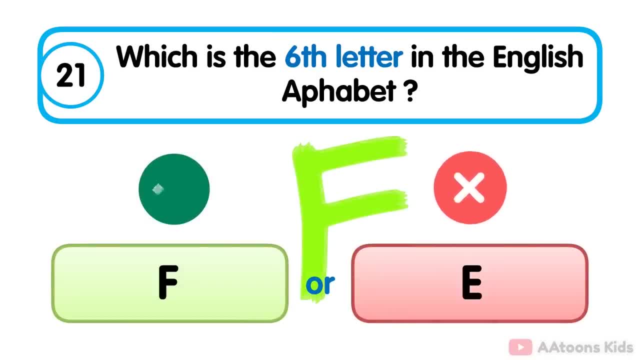 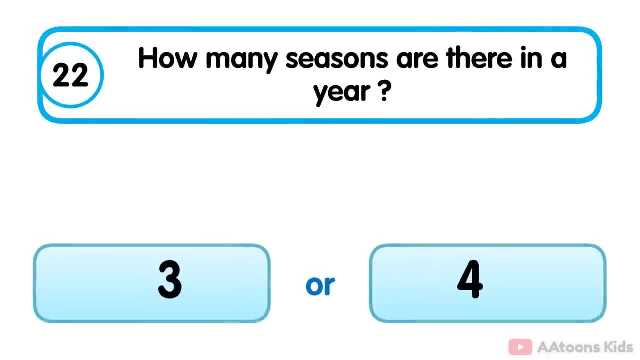 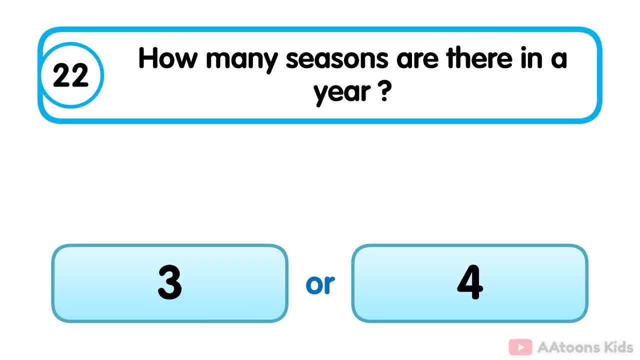 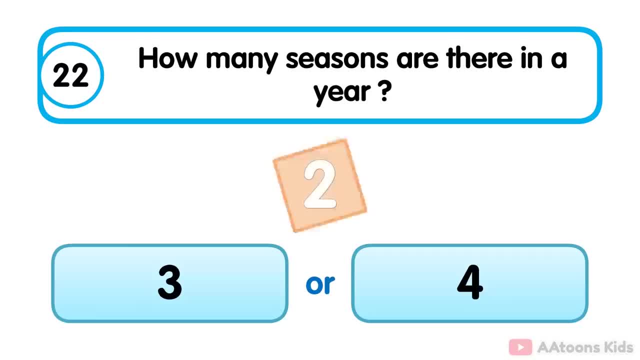 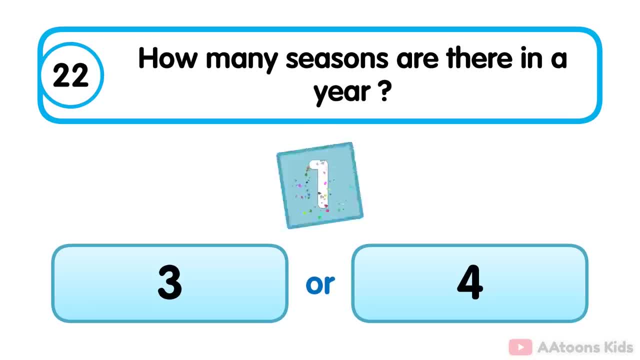 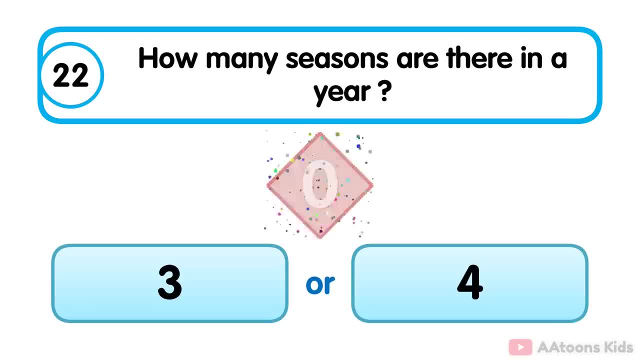 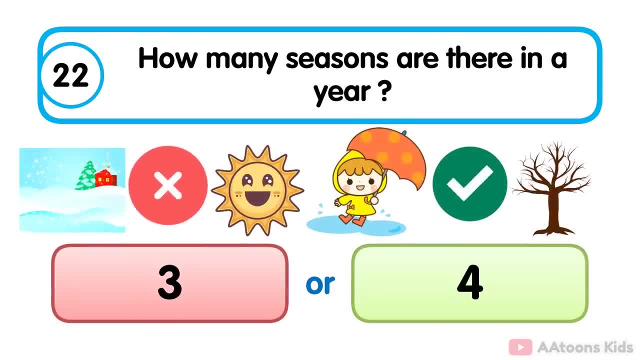 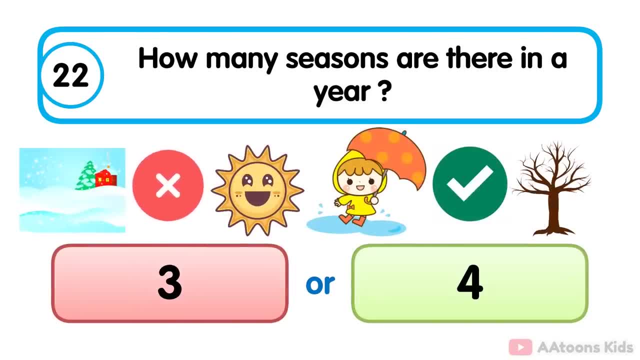 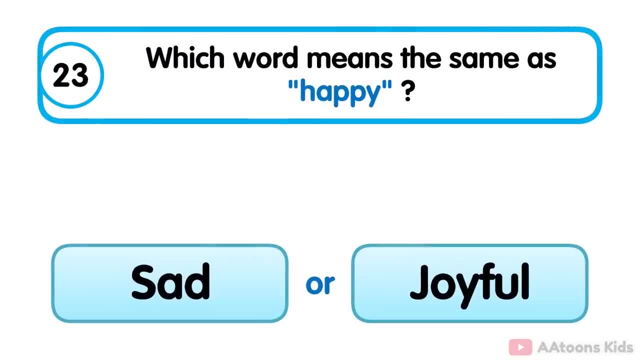 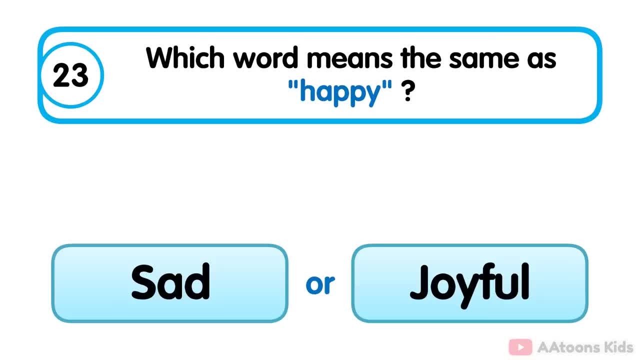 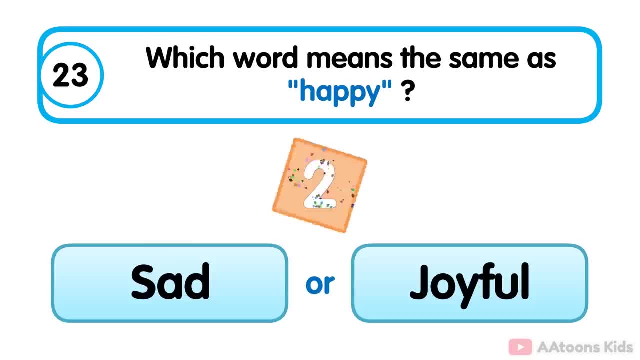 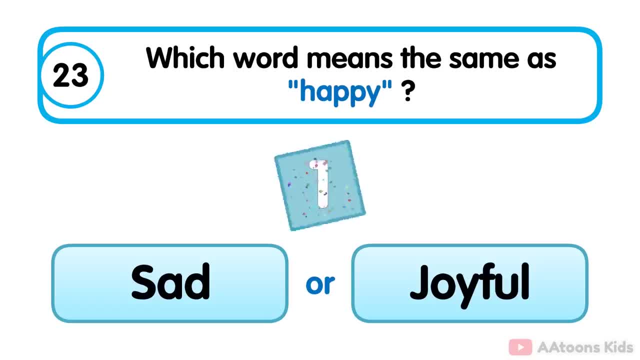 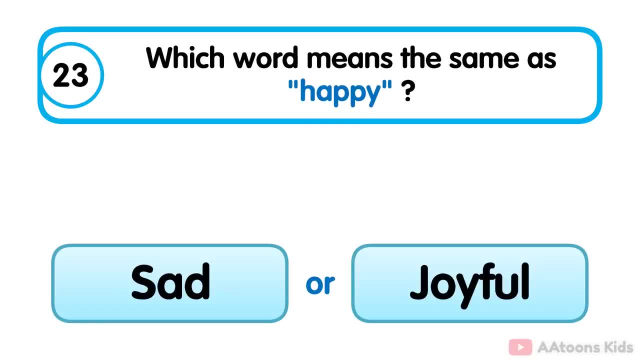 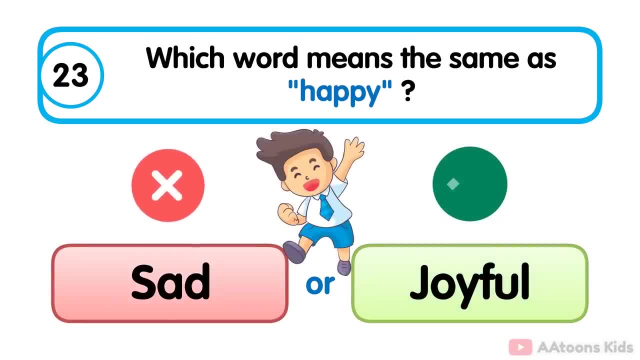 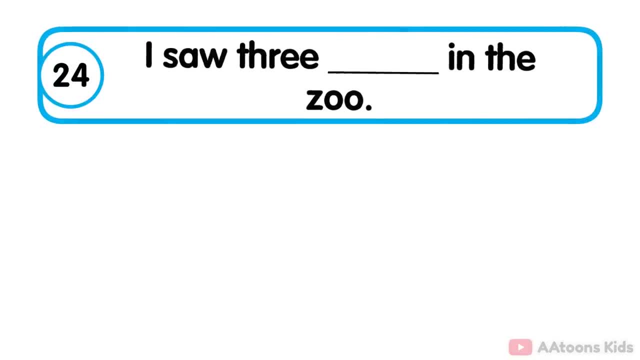 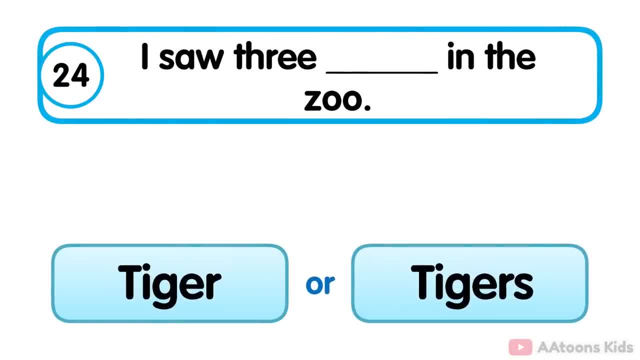 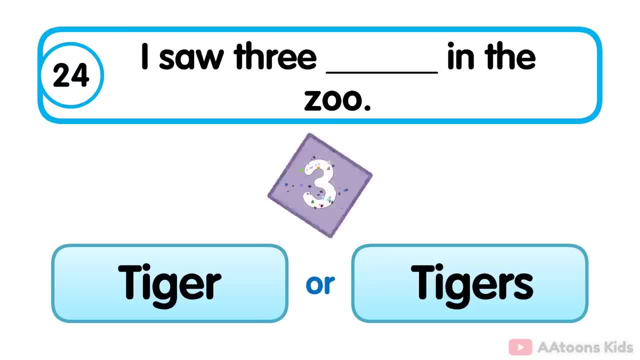 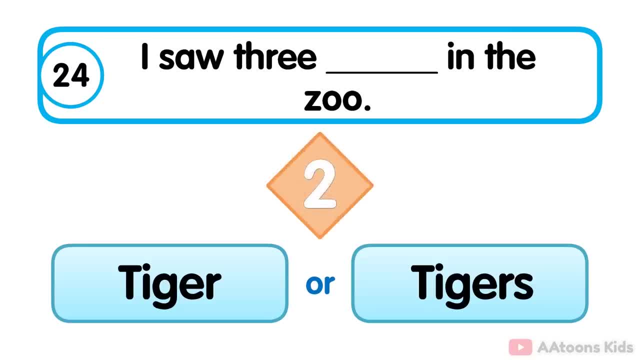 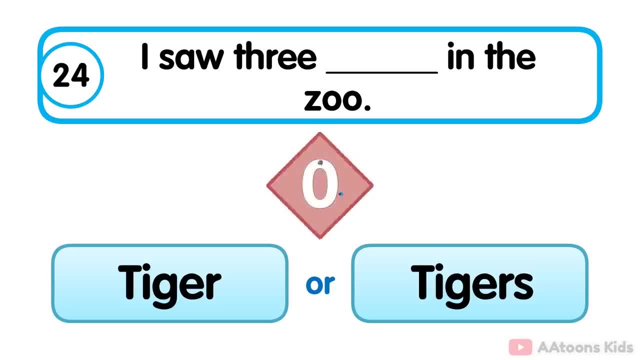 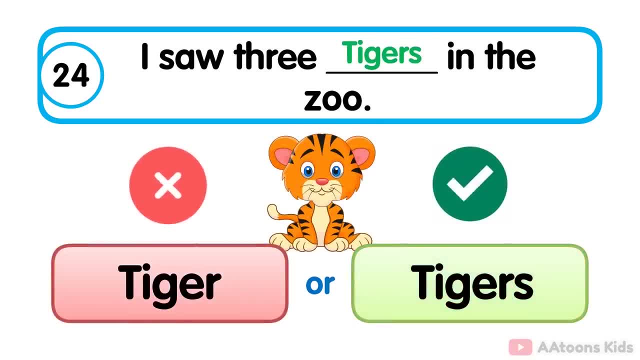 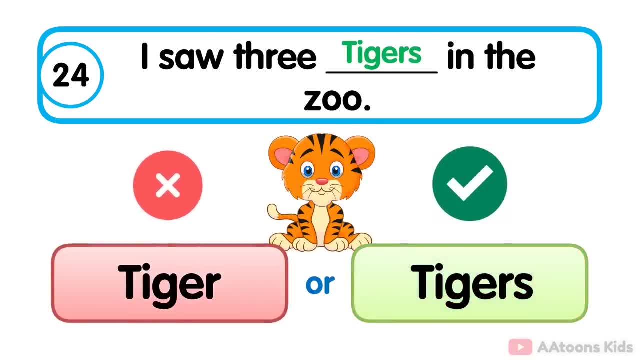 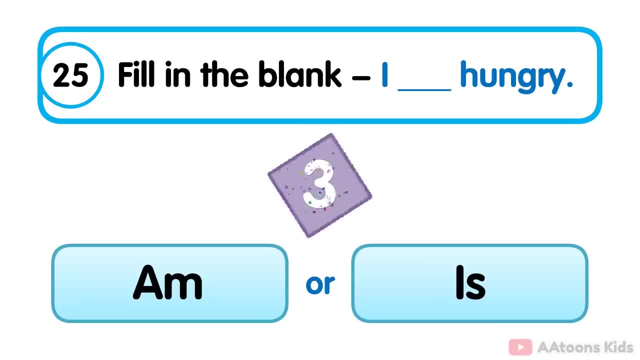 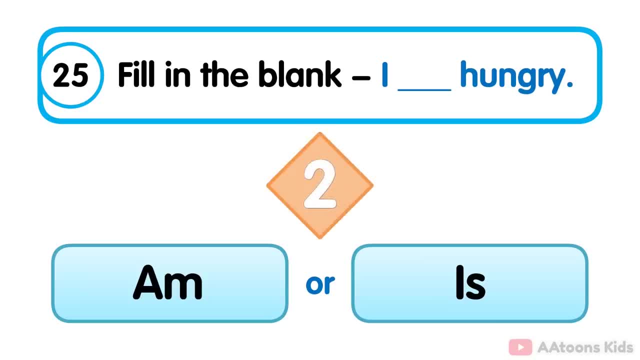